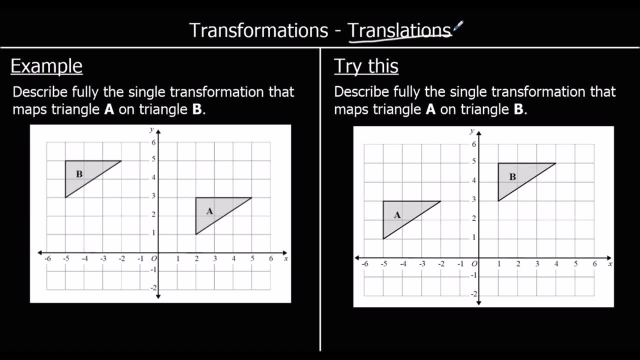 The first example here says: describe fully the single transformation that maps triangle A onto triangle B. So we're saying it's a translation, it's the same shape and it's just been moved. It's a translation, And how far has it moved? How far has shape A moved to get to shape B? 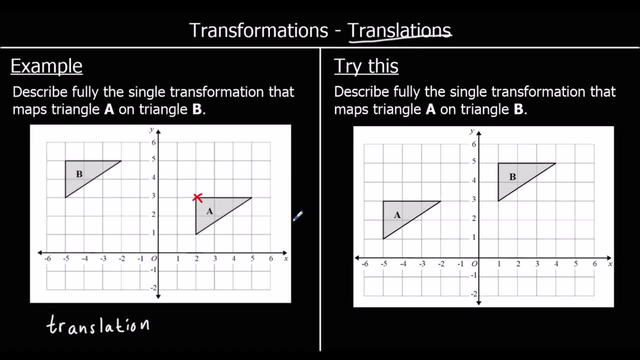 So if I look at this top left corner, I'm going to say it's gone 1, 2, 3, 4, 5, 6, 7 left and 2 up. So it's gone 7 to the left and it's gone 2 up. 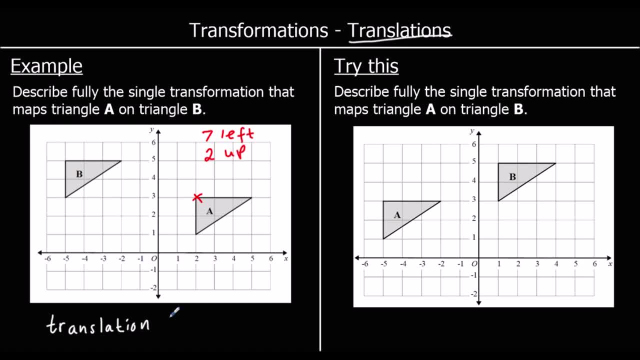 We can write this as a vector, So by the vector, And I write the change in the X on top. So it's gone 7 to the left, that's back 7 on the X axis, So it's minus 7, that's the change in the X and the change in the Y is up 2 spaces. 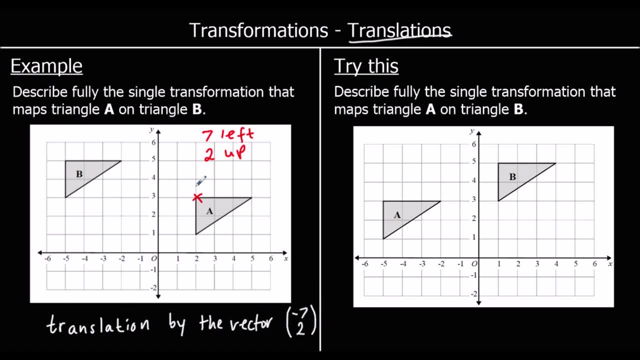 So it's a translation by the vector: negative 7, 2.. Back 7 on the X, up 2 on the Y. Back 7, or left 7, up 2.. Here's one for you to try So describe the transformation from triangle A to triangle B again. 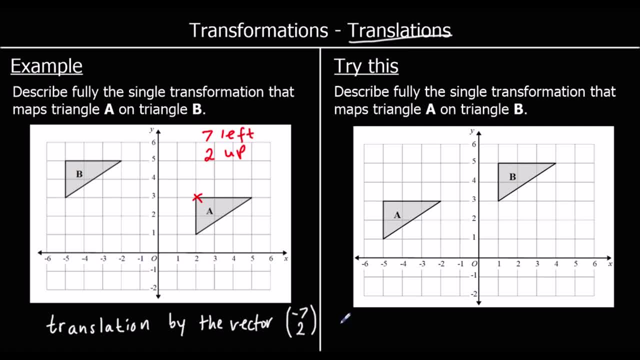 So again, We've got a translation. It's the same shape and it's been moved. So it's a translation. How far has it moved? So I'm going to use the top corner again. So how about the X, the change in the X? 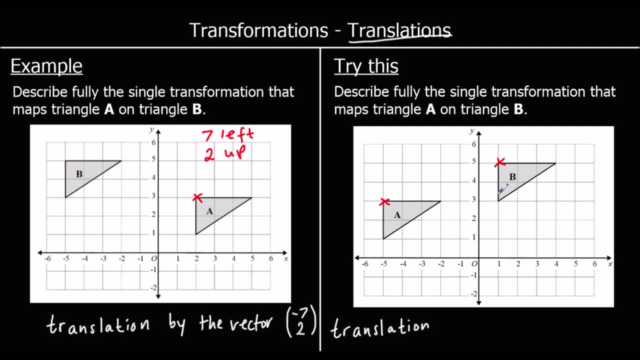 It's gone 1,, 2,, 3,, 4,, 5,, 6 to the right And 2 up. So it's a translation By the vector. So the change in the X is plus 6.. It's gone plus 6 on the X axis and plus 2 for the Ys. 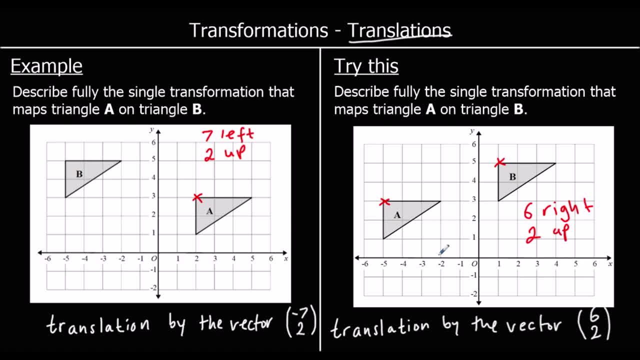 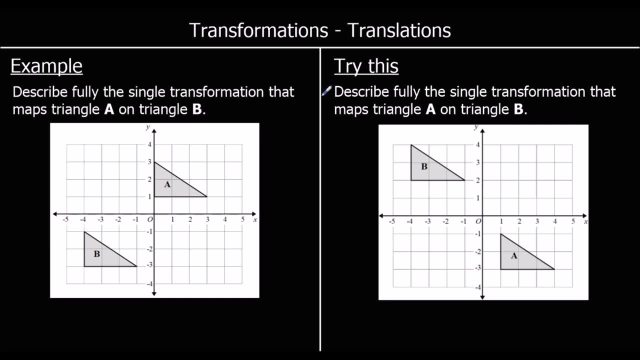 So it's a translation by the vector 6, 2.. Here's another question. So describe the transformation that maps triangle A onto triangle B. We're doing the same thing, So I'm going to take the top corner again, the top left. 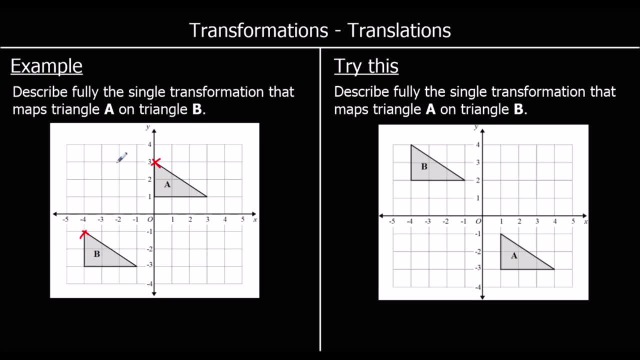 How far has it moved? 1,, 2,, 3, 4, left, That's minus 4 in the X direction, And 1,, 2,, 3, 4, down, Minus 4 in the Y direction. 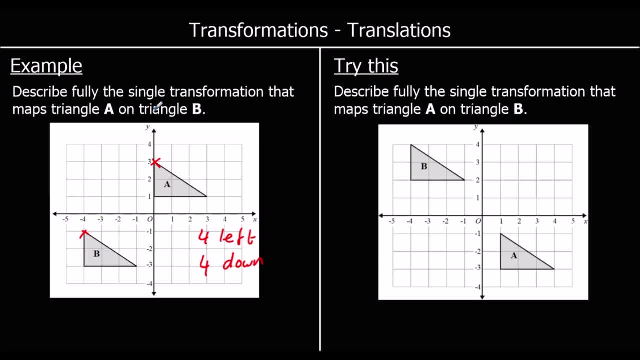 So minus 4 in the X and then minus 4 in the Y. So it's a translation. It's just been moved. It's just been moved By the vector, So 4 left, That's minus 4 in the X direction. 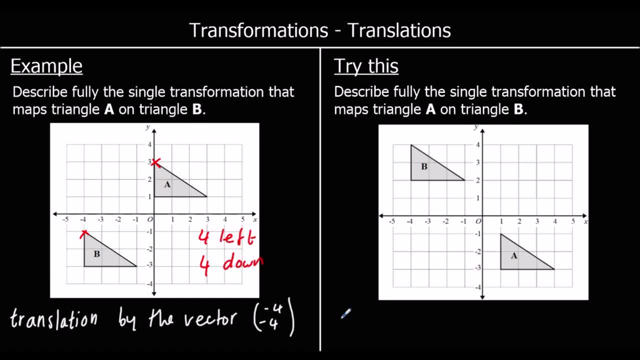 And 4 down minus 4 in the Y direction. It's a translation by the vector negative 4, negative 4.. And one for you to try. So give this one a go. So again, we've got a translation. 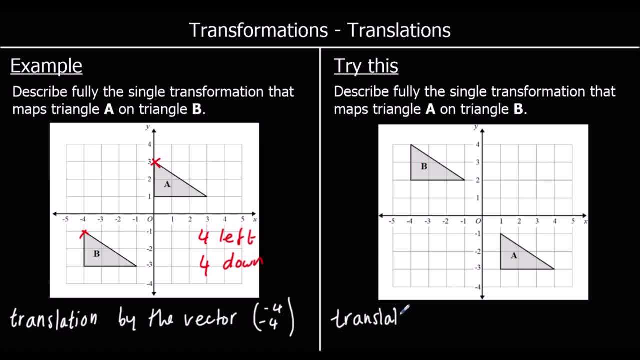 We've got a translation. We've got a translation And I'm going to put by the vector And then I'm going to work out how far it's moved. So pick the same point on both triangles. It doesn't matter which point you pick. 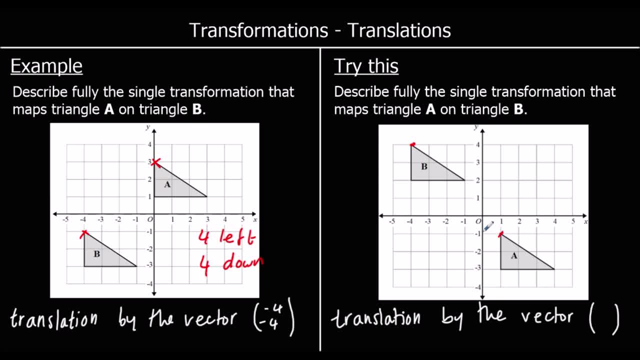 You'll get the same answer. So from A to B it's gone 1,, 2,, 3, 4, 5 left And 1,, 2,, 3, 4, 5 up, So 5 to the left. 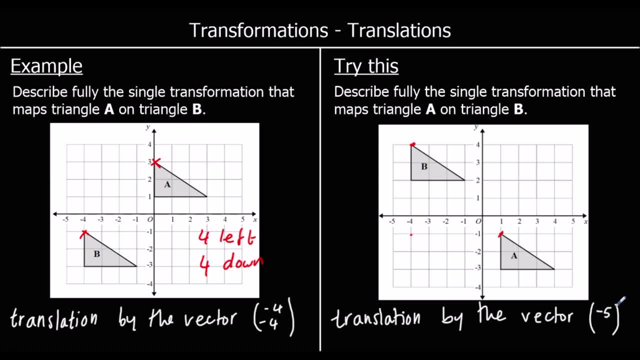 left is negative. 5 in the x direction. positive x is to the right, negative x is to the left and it's gone up 5, which is positive, 5 in the y direction. Positives are up, negatives are down. 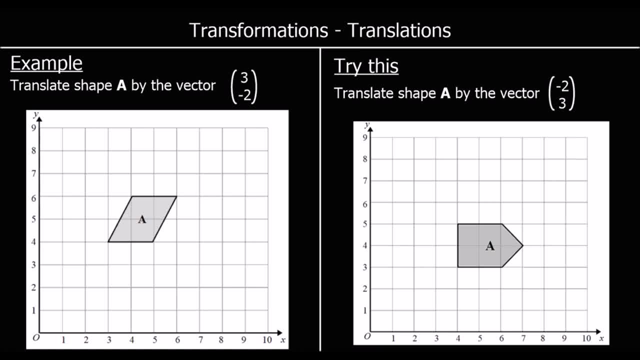 This is a different question. now We have to translate the shape, so we have to do the moving, So we need to translate shape a by the vector 3, negative 2.. So what does that mean? That's 3 to the. 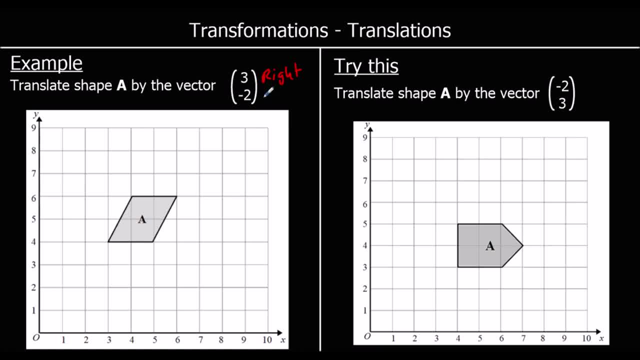 right and 2 down. So 3 right, 3 in the positive x direction and then down 2, so 2 in the negative y direction. So let's pick a point. I'm going to pick the bottom right. I'm going 3 to the right. 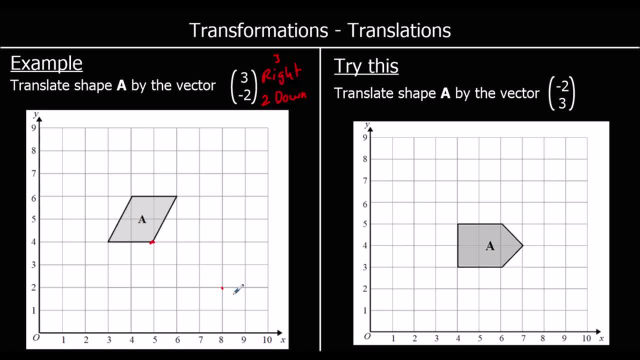 and 2 down. So that's going to be the bottom right of my shape, and then I could just draw it on from here. You could do this with every point, or you could just draw the shape on once you've worked out one of the points, It doesn't matter which one. 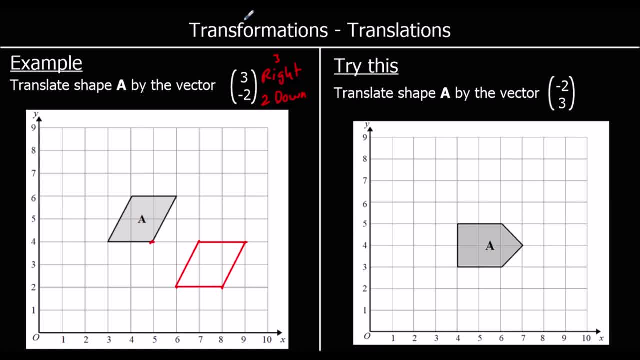 So I've drawn it on and I'll check with another point. So from the top, left, 3, right, 1, 2, 3, and 2 down, It gets me to there. So that is shape a, translated by the vector 3, negative 2.. 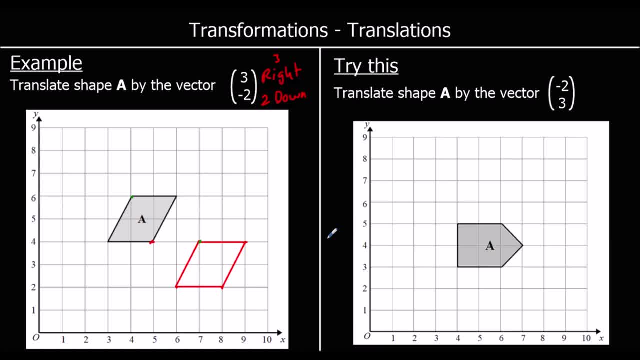 One for you to try. So give this one a go. So translate the shape by the vector: negative, 2, 3.. So that means 2 to the left, negative 2 in the x direction, 2 left and 3 up. 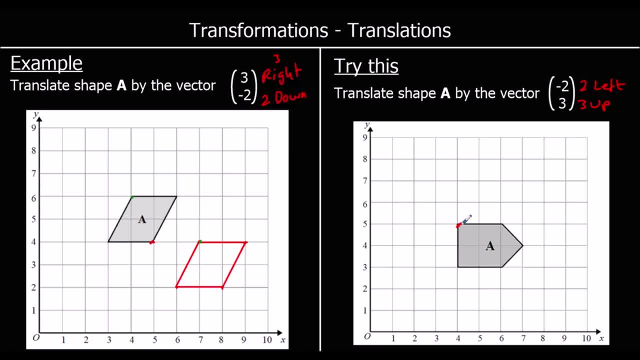 So let's pick a point And go 2 left and 3 up. So that's my top left corner And I can just draw the shape on And there is our shape. We can check with another point. So 2 left, 3 up. 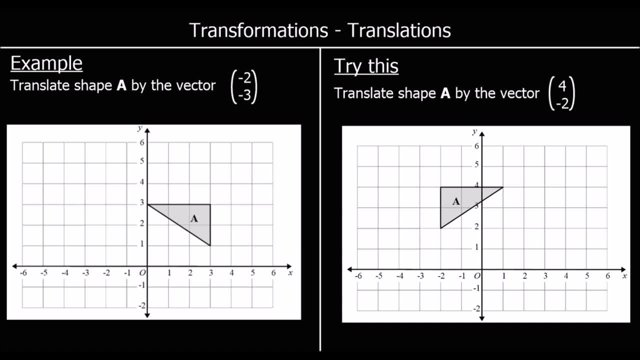 And another one of these. So translate shape a by the vector negative 2, negative 3.. So that's going to be 2 to the left, negative 2 in the x direction and 3 down, negative 3 in the y direction. 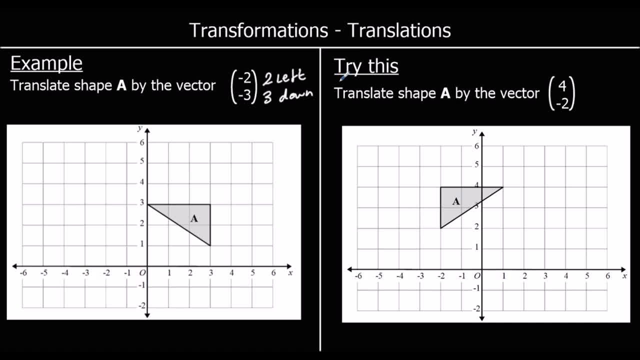 So negative in the x direction means left, positive means right, And in the y direction positives up and negatives down. So we're going 2 left, 3 down. So pick a point, Go 2 left, 1,, 2,, 3 down. 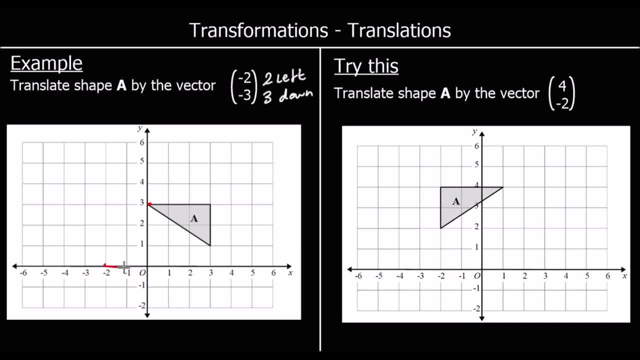 And then we can draw the shape on. So it goes 3 along the top, 2 down. So that's our triangle And I'll check with another point. So 2 left, 3 down, And it should work for all points. 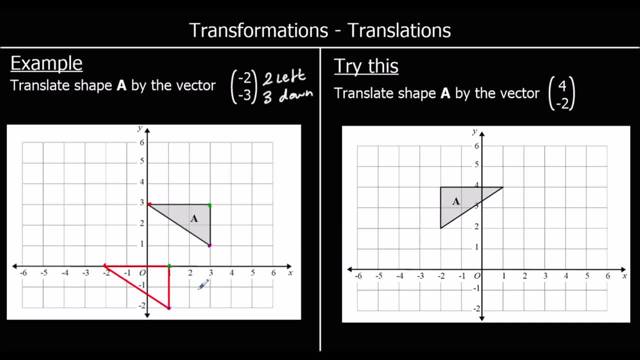 2 left, 3 down. Okay, one for you to try. So translate shape a by the vector 4, negative, 2.. So 4, negative 2 means 4 to the right, positive, 4 in the x. 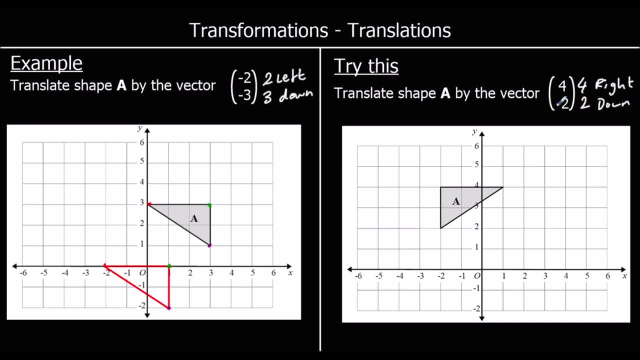 and 2 down, negative 2 in the y direction. So we're going to go 4 to the right, 1, 2, 3, 4, and 2 down. So that's the top right. So it goes back 3.. 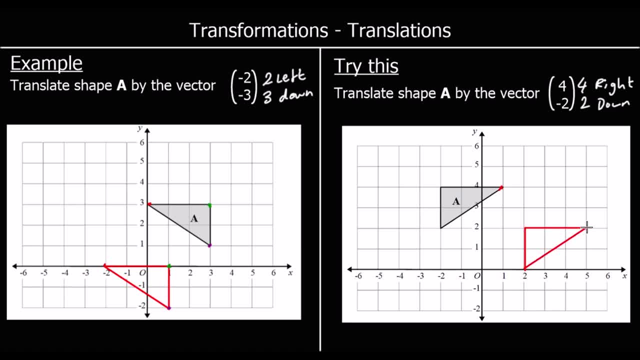 Down 2.. And join up the triangle And we can check with another point. So 4 right, 1,, 2,, 3,, 4, and 2 down, 4 right, 1,, 2,, 3,, 4,, 2 down. 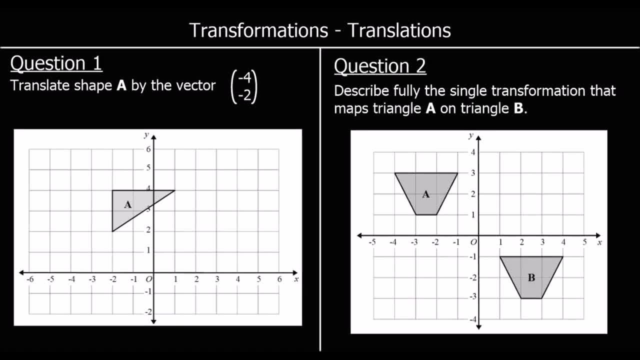 Okay, 2 questions to finish up. So give these ones a go. Question 1 says: translate shape a by the vector 4, negative 2.. So give these ones a go. Question 1 says: translate shape a by the vector 4, negative 2, in the y direction. 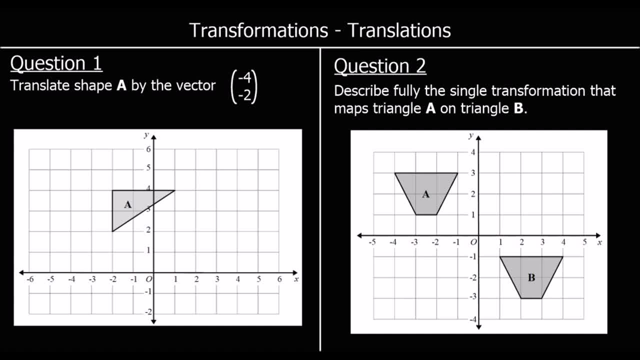 So it goes back 3.. Question 1 says: translate shape a by the vector 4, negative 2 in the y direction. so it translates shape a by the vector negative, four negative two. so negative four negative two. so the top one's the x, change the change in the x. so it's going four left, so positive is right. 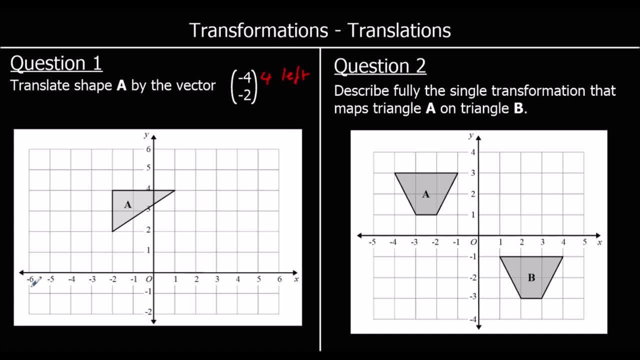 where the positive x numbers are and negative is left, and for the y change. positive means go up, negative means go down, so it's two down. so we're taking any of the points and moving them forward to the left and two down. and if we did that for every point, 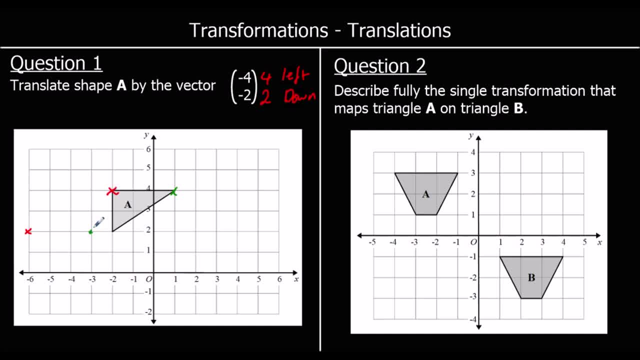 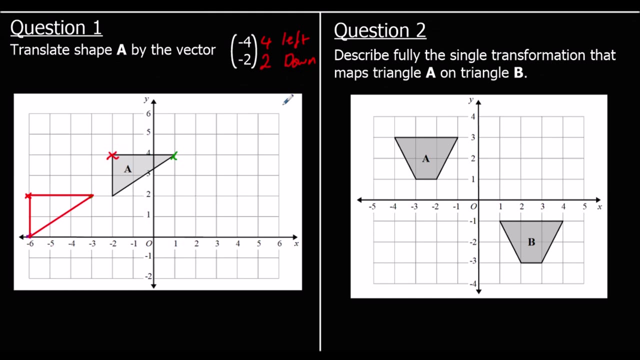 so one, two, three, four, one, two, one, two, three, four, one, two, one, two. we would make our triangle and question to describe fully the single transformation that maps triangle a onto triangle B. so it is a translation and I'm going to write by the vector and then I'm going to figure out how far it's.